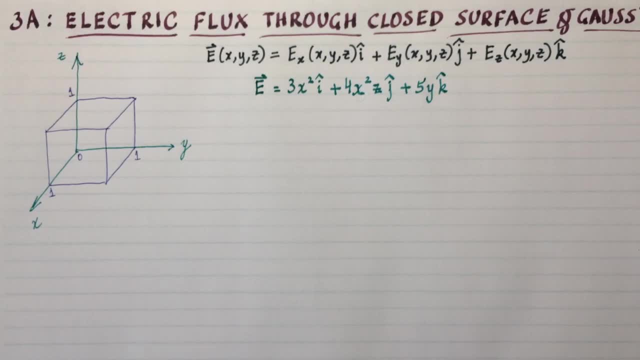 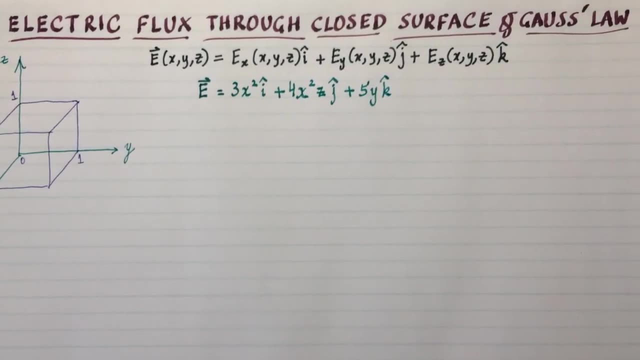 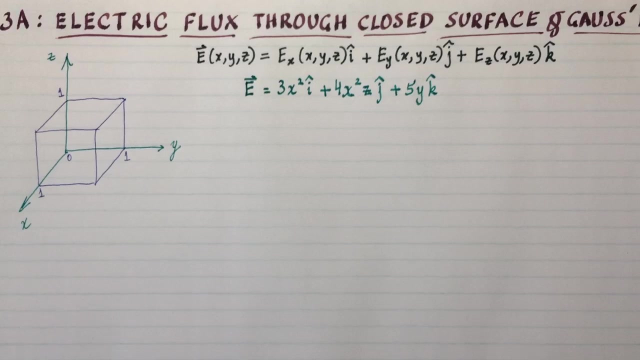 I will begin my discussion of electric flux through a closed surface and Gauss's law by a simple example of trying to find the electric flux through a closed surface, namely the surface of the cube pictured here of side 1.. Electric fields can be very complicated. The most general expression can have all three functions of x, y and z, and the x component, y component and z component themselves can be different functions of x, y and z. 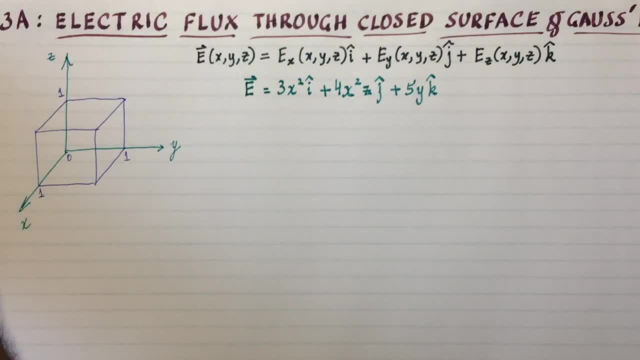 The example I'm choosing is a much simplified version of the most general possible electric field. The x component is 3x squared, the y component is 4x squared z and the z component is 3x squared z. The z component is 5 times y. 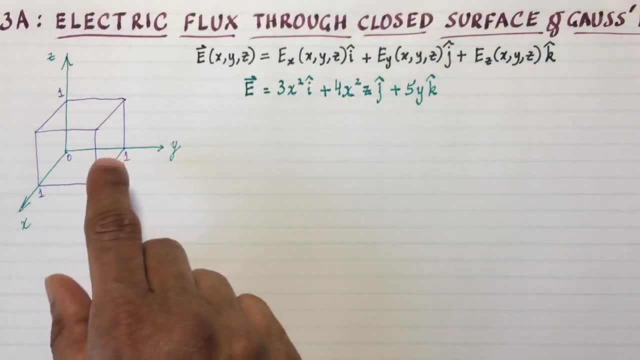 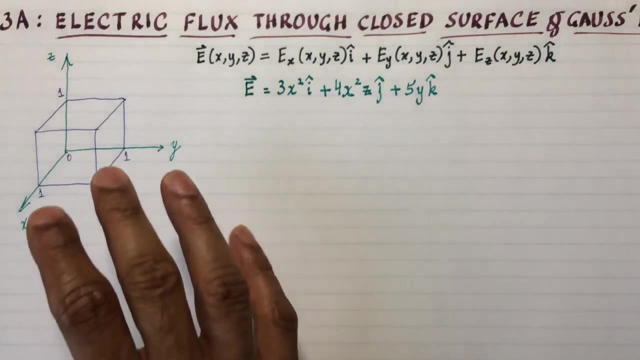 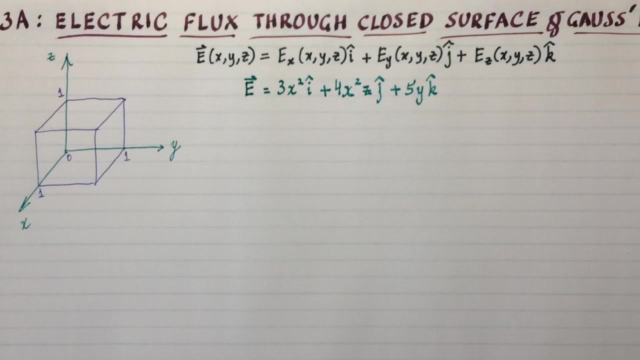 We have to take this electric field and find the flux through the surface. Now, if you want to think about the flux in a physical way, you can think of a fisherman putting a net inside a pond and finding out, at the end of the day, how much fish he or she has caught. 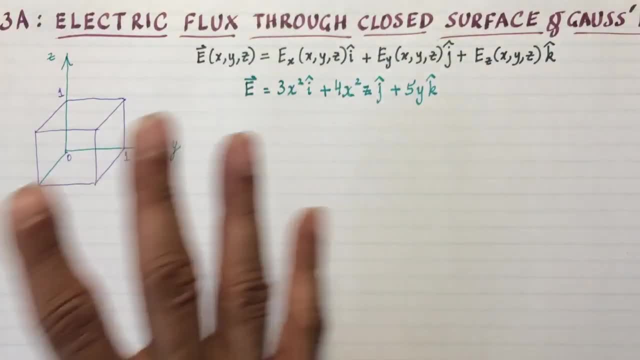 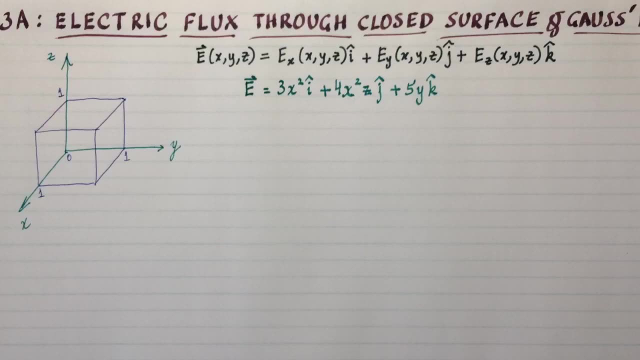 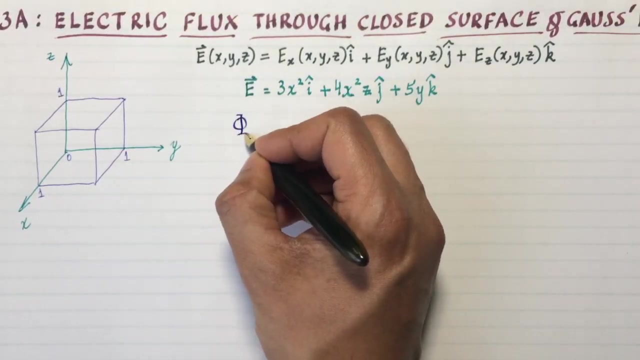 So the electric field can be thought of as little fish darting around the pond. Okay, so we have to find out what the net is, What the net catch of this fisherman is. The catch is measured by the concept called electric flux, and the flux is given as follows. 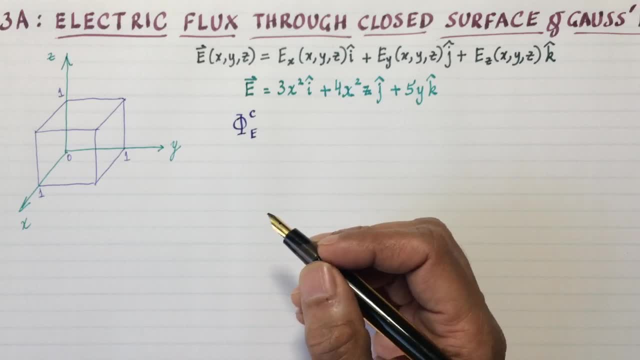 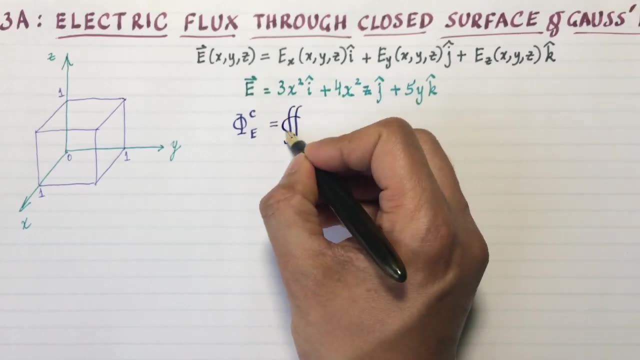 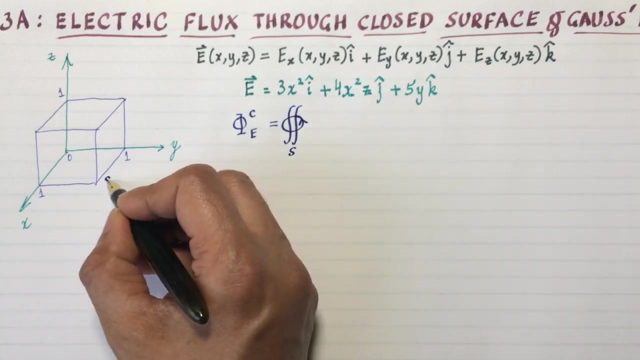 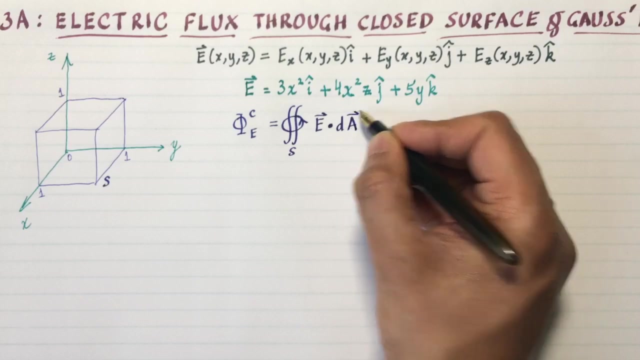 The electric flux through a closed surface, denoted by phi, sub e, superscript c is the oriented surface integral and that circle with an arrow means it's an oriented surface integral over the surface, in this case the surface of the cube of the electric field dotted with the area vector on the cube. 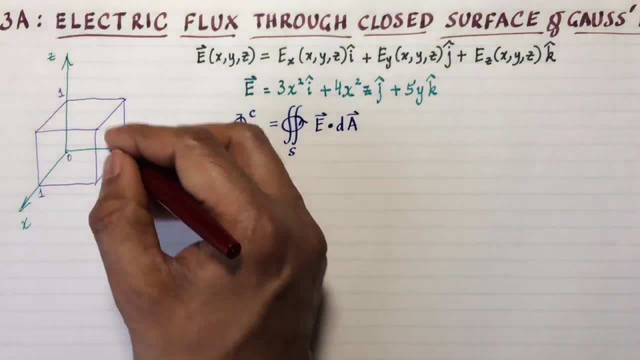 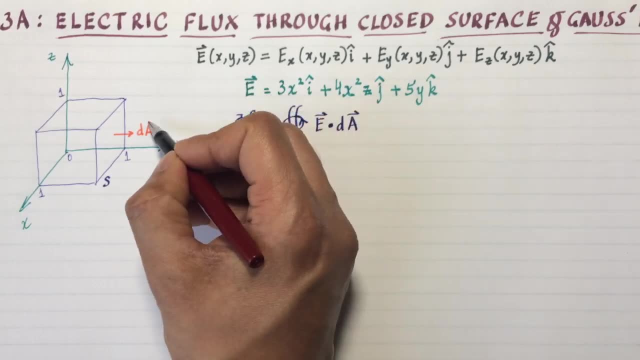 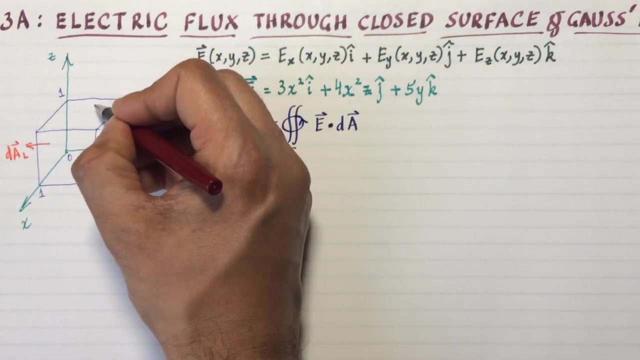 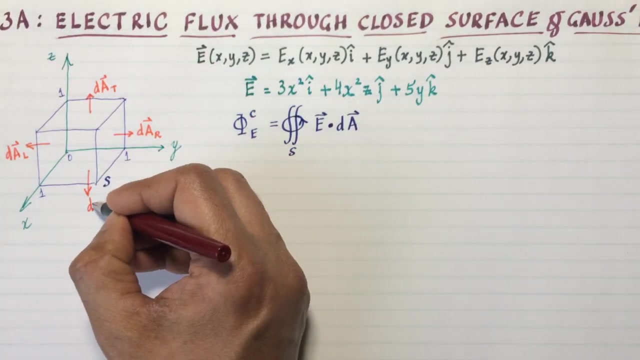 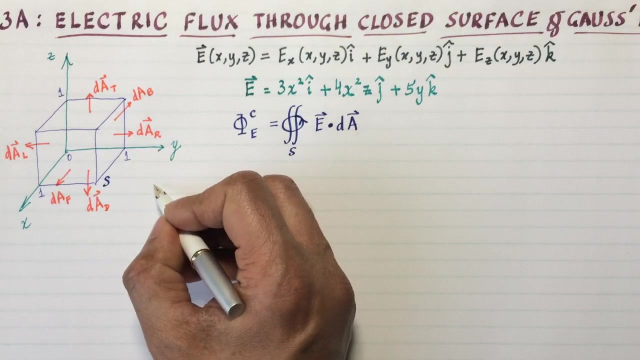 There are six area vectors on this cube. I will denote them by da right, da left, da top, dA down, dA front and dA back. It's not too hard to write actual vector expressions for all these dA vectors, which I will do next. 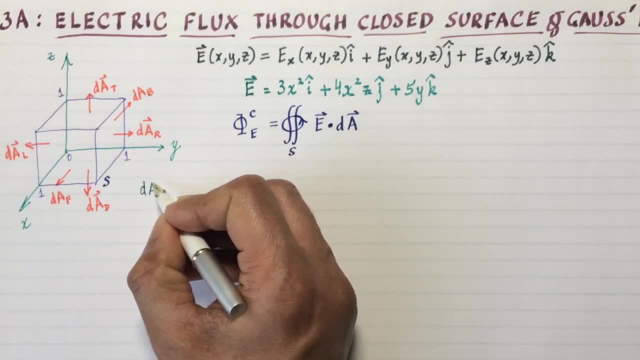 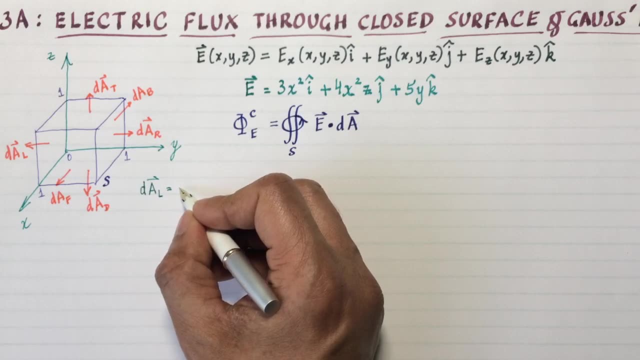 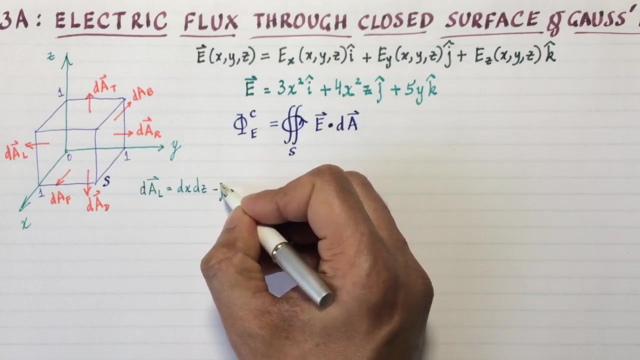 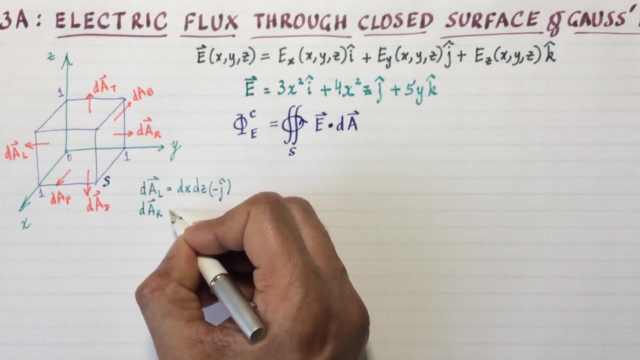 First, dA left is just going to be because it's on the surface, with x and z coordinates. it's just going to be dx, dz times, negative j hat because it's in the minus y direction. dA r: once you write one expression, the other one can be written almost immediately. 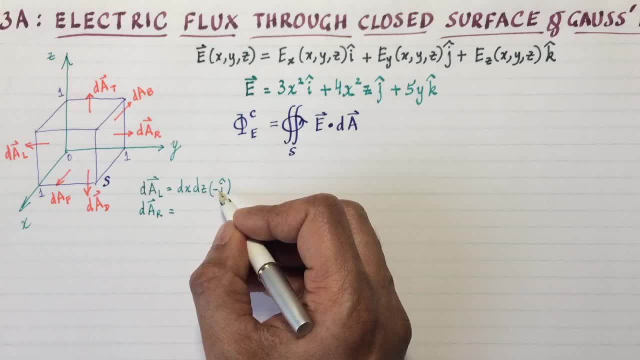 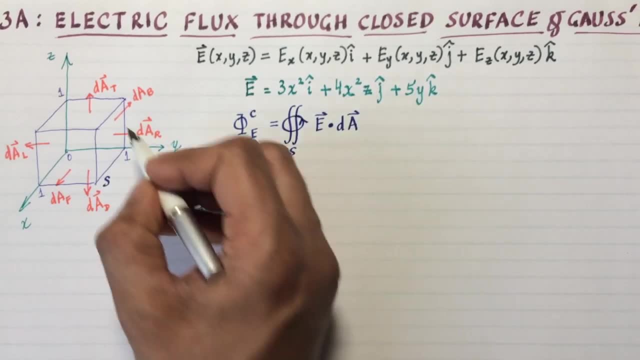 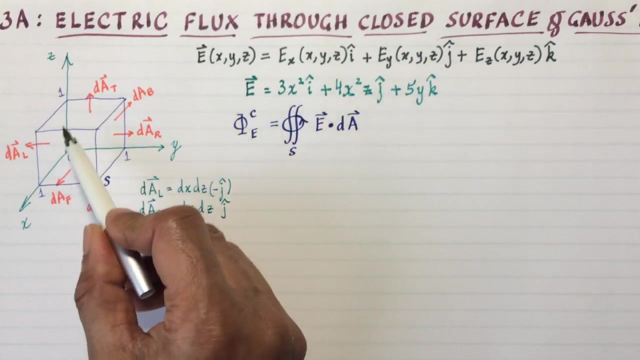 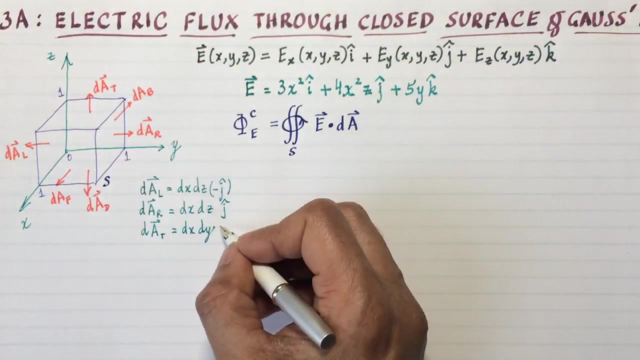 The opposite vector can be written almost immediately. You are just removing this minus sign and substituting a plus sign, So let's repeat this performance for dA top. next dA top is going to have coordinates x and y, so it's dx dy in the direction z, so that's k hat. 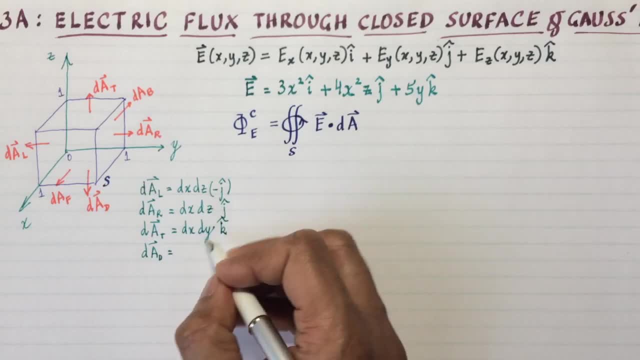 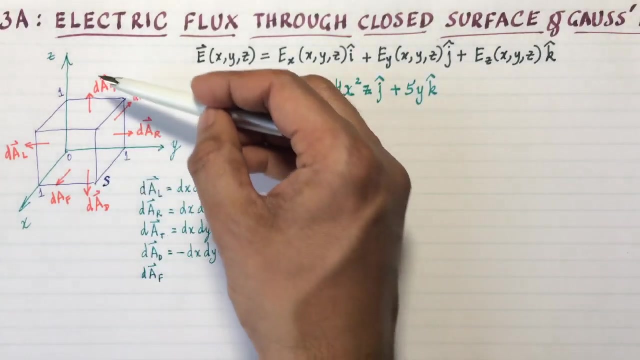 And dA down will then be the opposite of that, which is negative dy. So it's going to be x dy, k hat. And lastly, we have dA front and dA back. So dA front. now the front and back surfaces are in the yz plane. 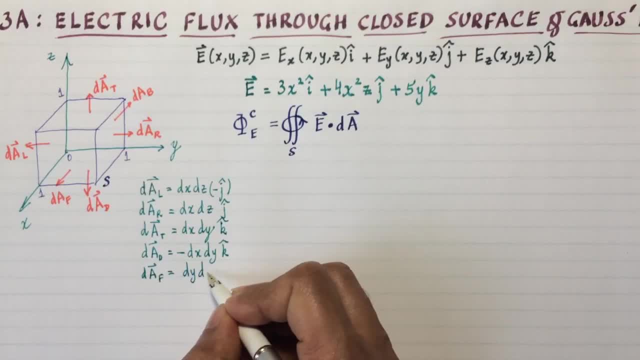 So that's going to be dy dz in the x, which is i hat, And dA back is the same thing, But in the negative i hat direction. once you've written all these dA vectors, you just then have to split this up into six integrals and do each one to find the flux. 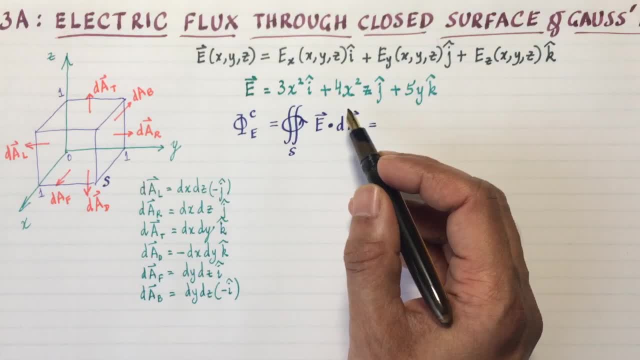 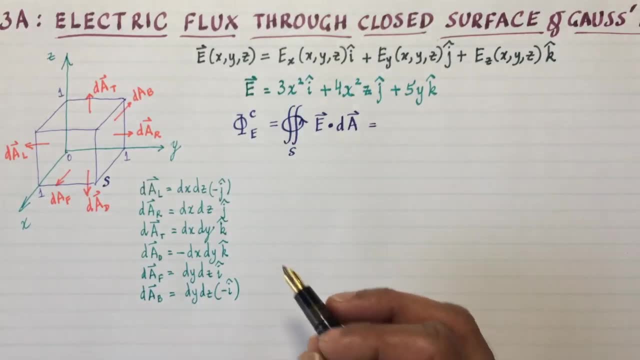 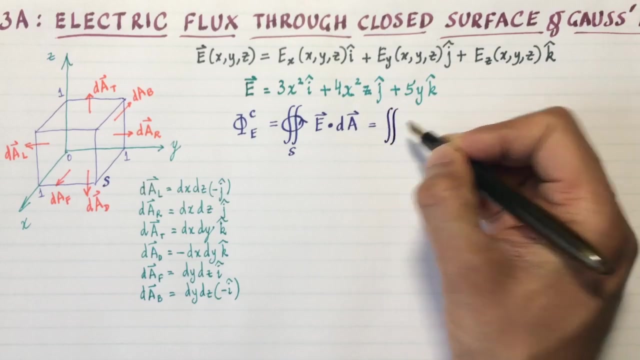 Now don't be too worried. I have pre-arranged this to only have one contribution, and that is in the flux through the the front side. So let's try this: Once you split the double integral into pieces, you're not going to put the closed sign anymore. 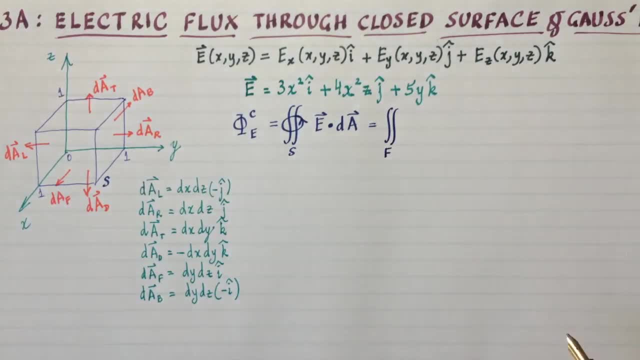 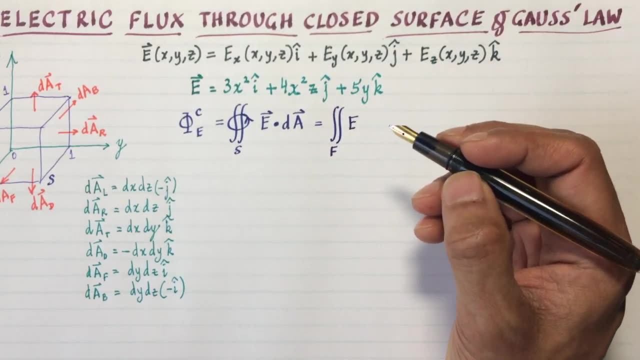 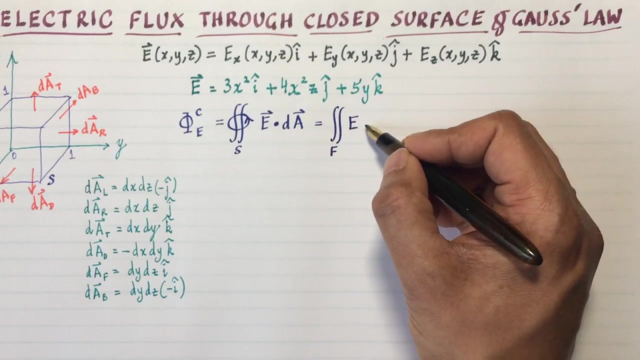 Closed means the entire cube and this means each face of the cube. So the front face of the cube times remember dA front- is the i hat. So when I take the dot product, the only term that will survive is the x component. 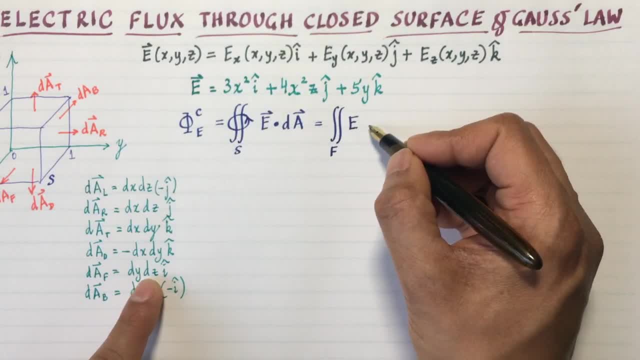 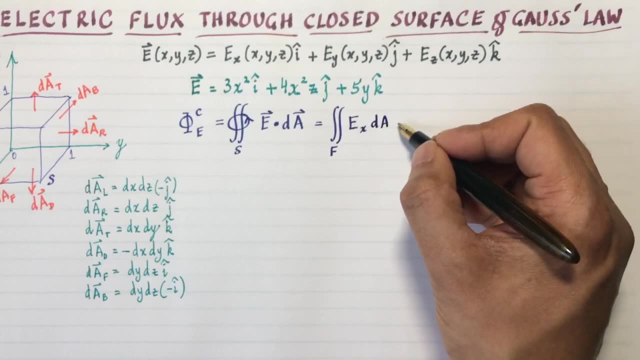 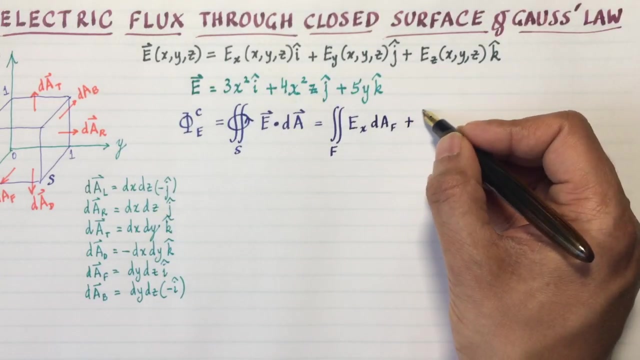 And the i hat component. So this is going to be e sub x times dA front without the i hat plus the integral on the back of the x component at the front location. This is at the front location here: x component at the back location. 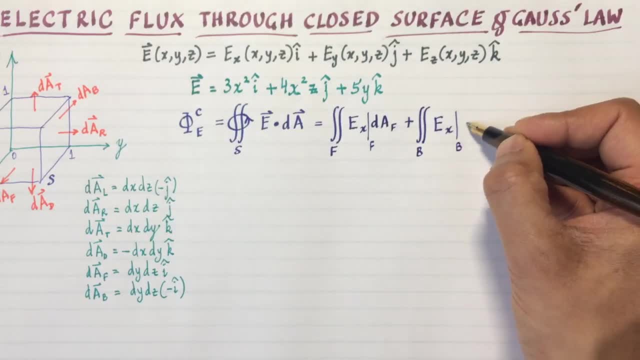 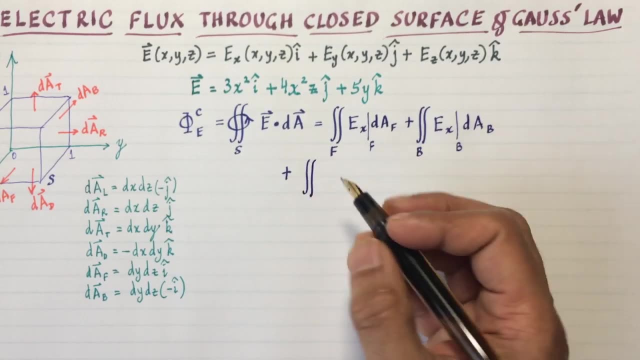 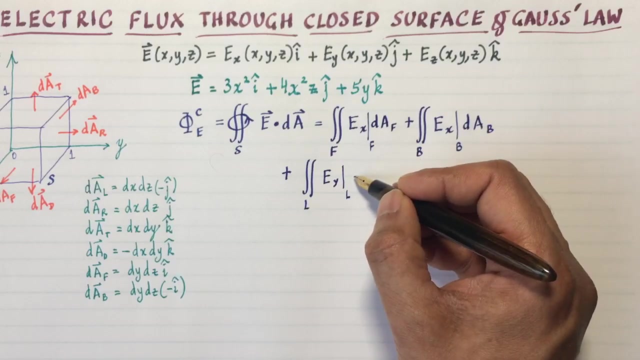 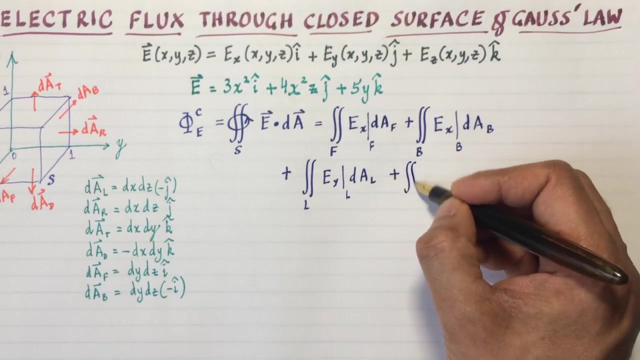 x, dA back, And then I'll have terms for the other sides. Let me do left. Left will involve the y component, So that's gonna be ey evaluated at the left side times, dA left plus right, which would be EY evaluated on the right side times, DA right and then two. 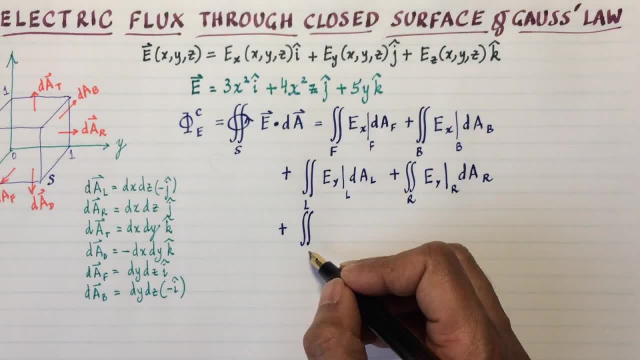 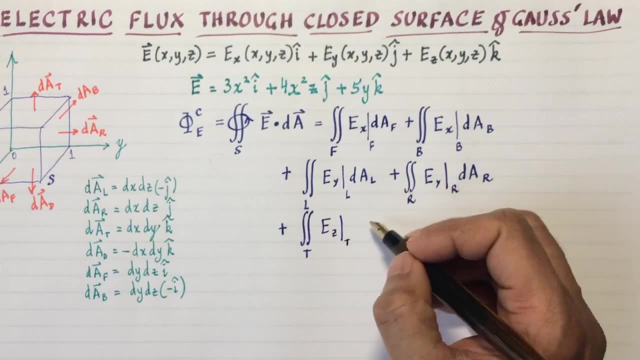 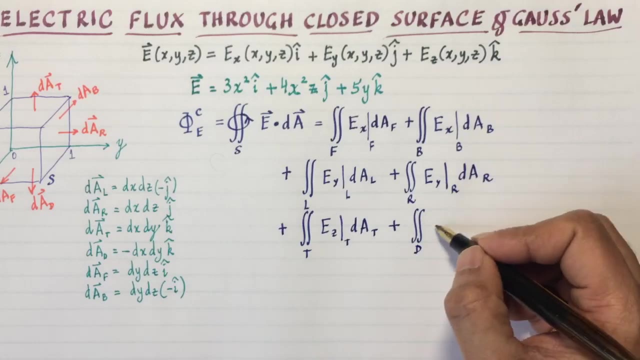 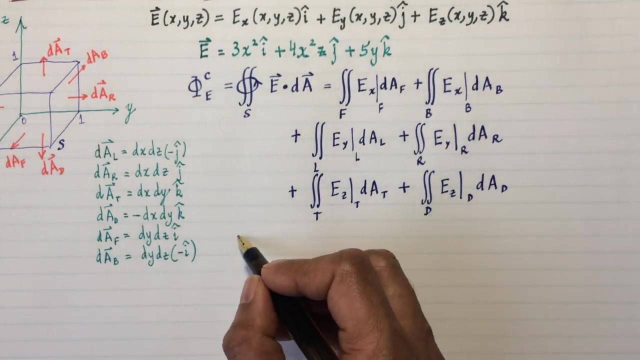 more terms, which would be top and down. Tops and downs refer to the K component, so it's: EZ evaluated at the top side times- DA, top plus down. EZ evaluated on the downside, DA- down. Now we just have to write these integrals out one by one. 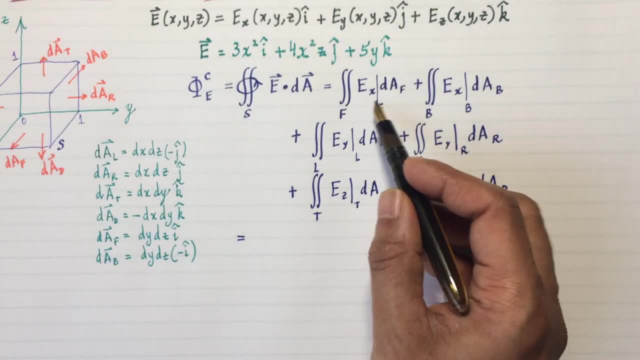 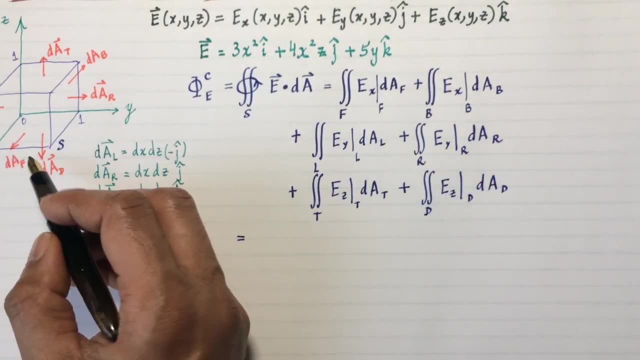 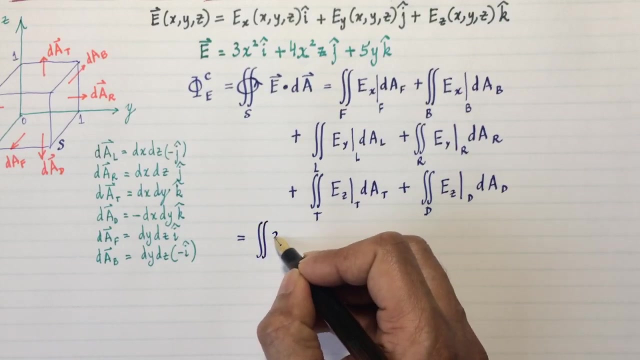 So this is just a very routine procedure. EX is 3X squared Evaluated at the front surface, means evaluated at X equals zero. It's one. So 3X squared evaluated at X equals one, is just three. So that's going to be three times DAF, which is DYDZ. 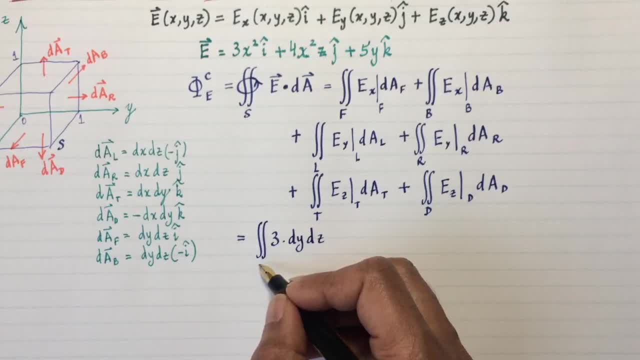 Now the limits of all these integrals are from zero to one. Each of these integrals goes from zero to one on the respective variables. For example, this integral is DY from zero to one. That integral is DZ from zero to one. 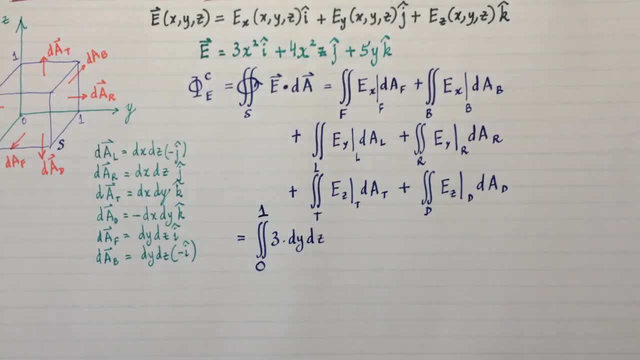 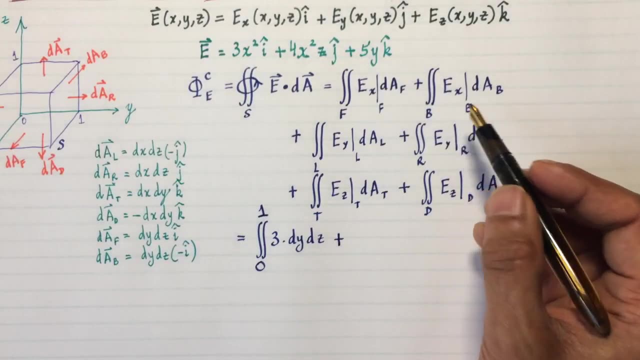 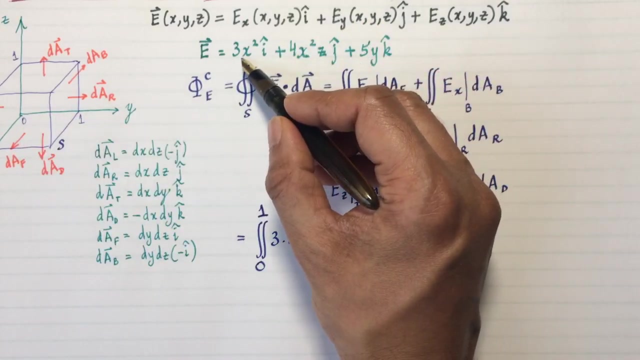 To avoid writing it twice, I'll just put a big fat zero and a big one. What about the back surface? On the back surface, which means X equals zero, EX is zero because it's 3X squared. That's just zero. 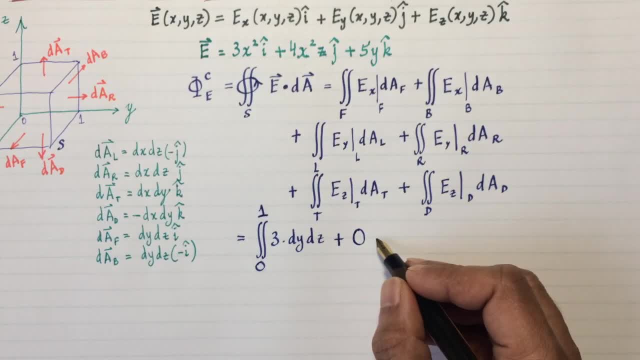 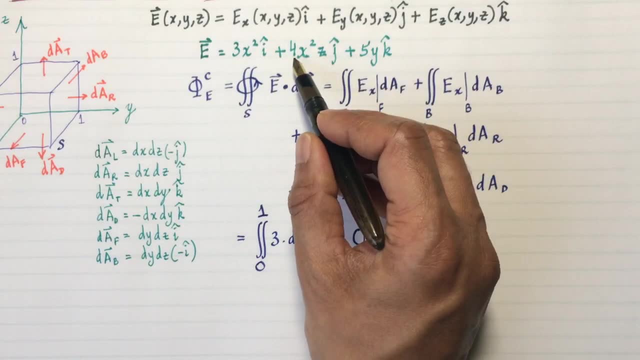 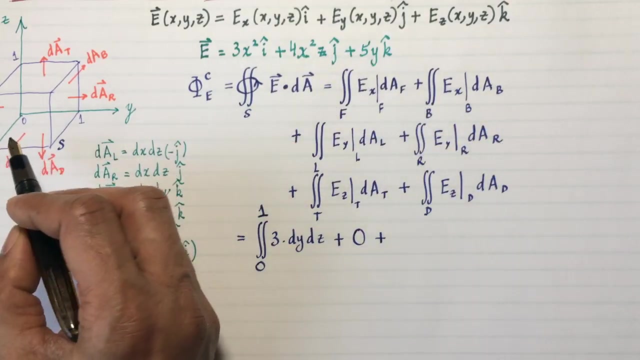 Very nice, That integral is easy. Let's do the next integral: E left, EY. EY is 4X squared Z, And the left side is at Y equals zero. Well, you're out of luck. Y equals zero does not occur there. 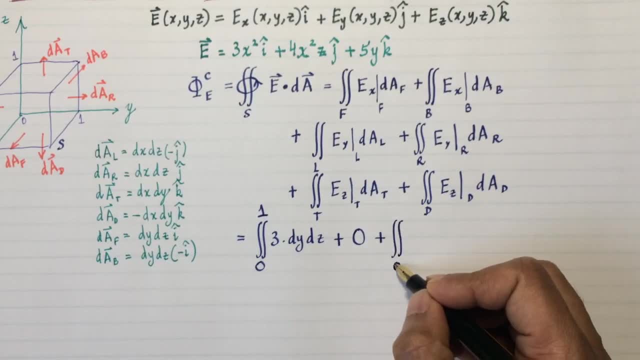 So you have to do a full blown integral zero to one, big zero to big one of 4X squared Z times DAL, Which is negative, DX, DZ, Because you look at the DAL there, it's got a negative sign. 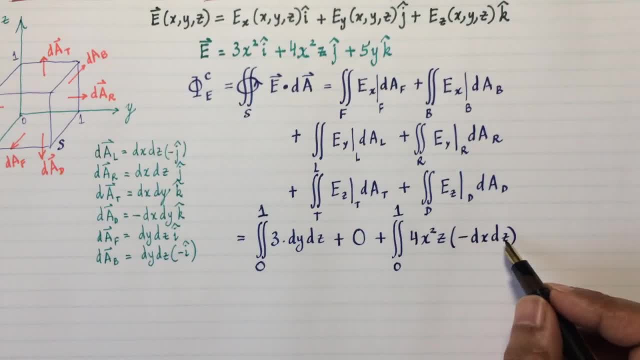 We don't have to worry about doing this integral. You can actually do it if you want, or put it in Wolfram alpha, or do the double integral if you like. But you don't have to. I'll tell you why soon. 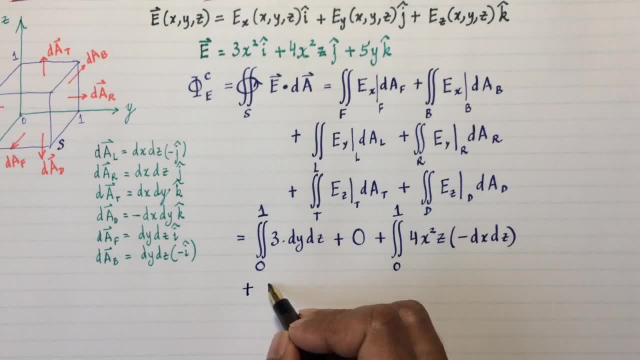 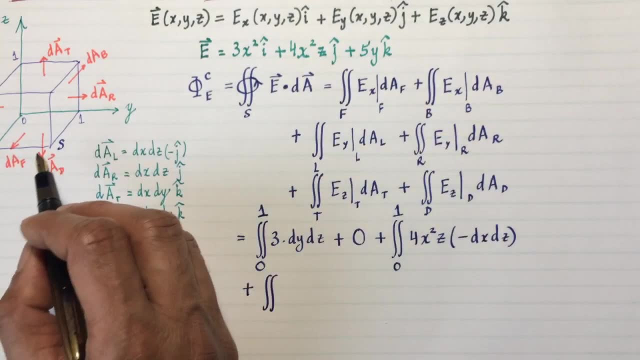 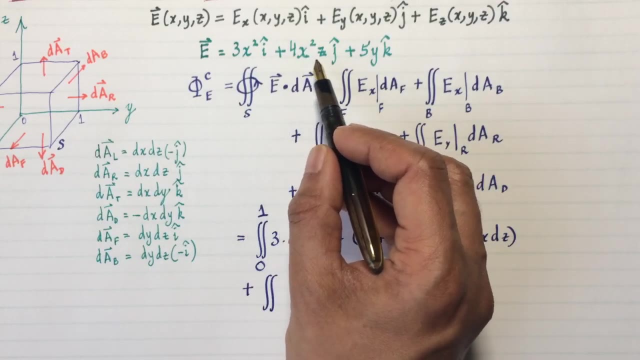 Let's look at the other integral. That one's going to be the same integral on the right side. Now EY, Y, X squared Z on the right side still does not depend on Y, So it's still going to remain as 4X squared Z. 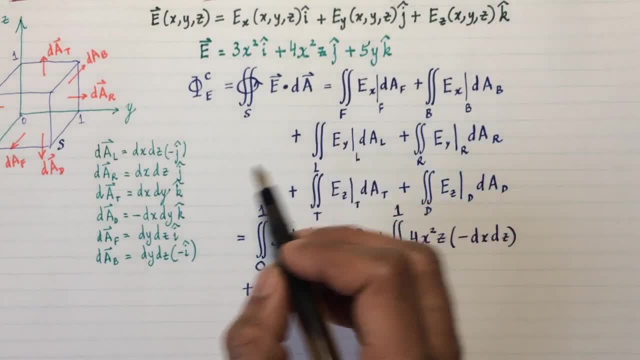 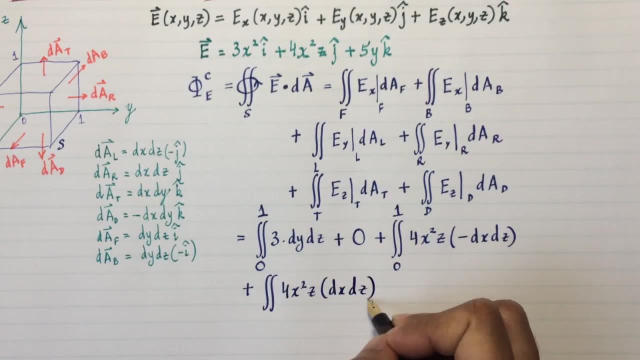 But on the right side, DAR is DX, DZ, Big zero to big one. And now you see why you did not have to worry about doing this integral, because they simply cancel out, And you can expect cancellations here too. Let's try this out. 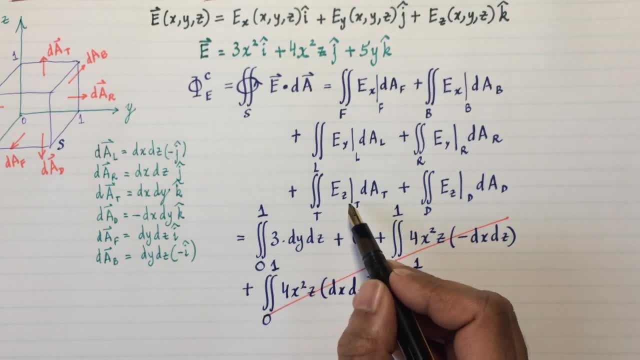 So this will be integral. big zero to big one. EZ is 5Y At the top, it remains 5Y. At the bottom also, it remains 5Y. So that's going to be 5Y. The top integral involves DX, DY. 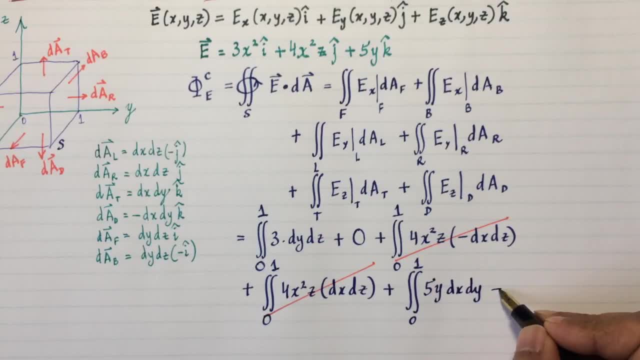 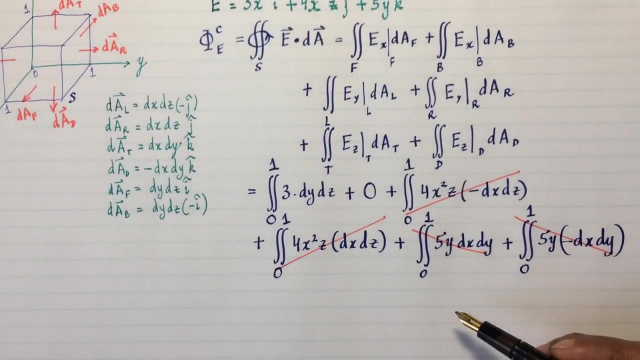 This integral is the same thing: big zero to big one, 5Y, but with a minus DX, DY. So these two integrals also cancel out. The only serious integral that needs to be done is the first integral. 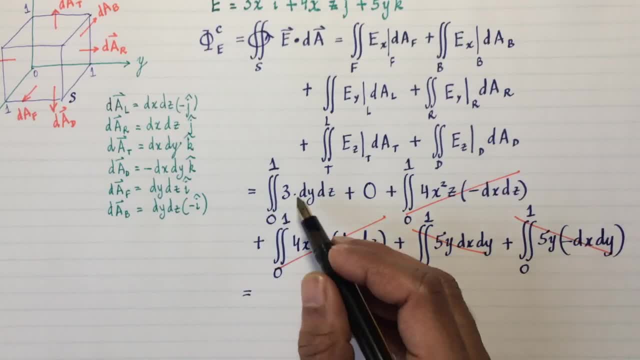 Fortunately for us, that's a very simple integral. A 3 can be taken outside. The integral of DY is just Y. It should lose the box And for theiz, the law of logic says that A can not be taken outside Y. 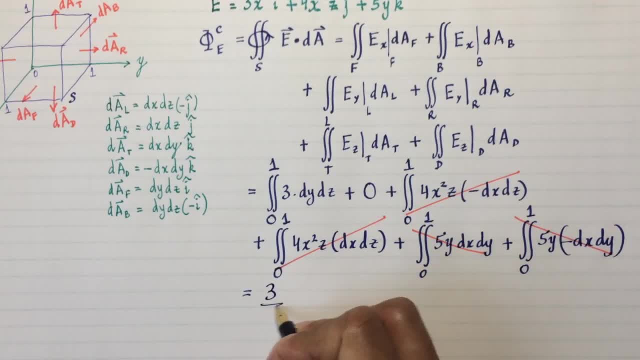 Because this physical integral is sự. So everybody works out how right this can come out. You can perform calculations and learn yielding. You can shape these in 양 and umm. So what we're doing here is we're going to put one integral inside Z and divide it. 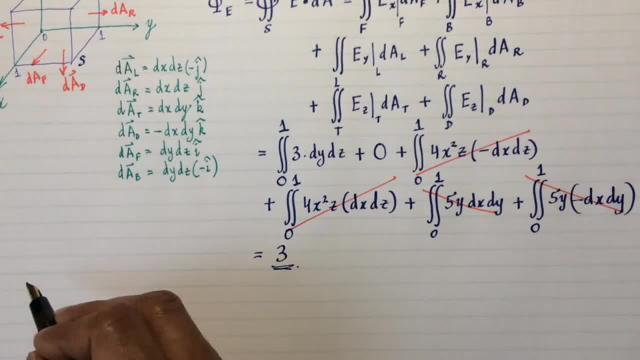 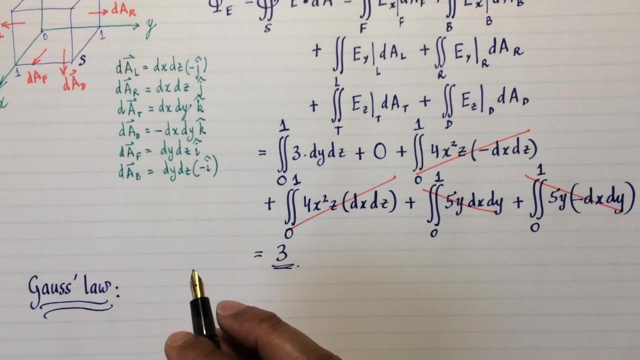 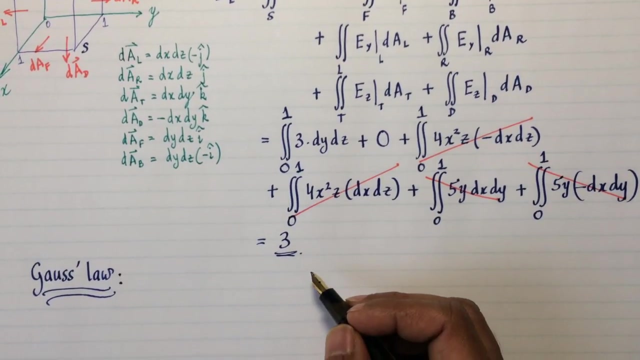 by one in Y related to one, So it becomes zero. Two integrals: flux you catch in your net and what kind of charge you have in that net. So it's as though, without looking into the net, you can say what kind of fish you caught. 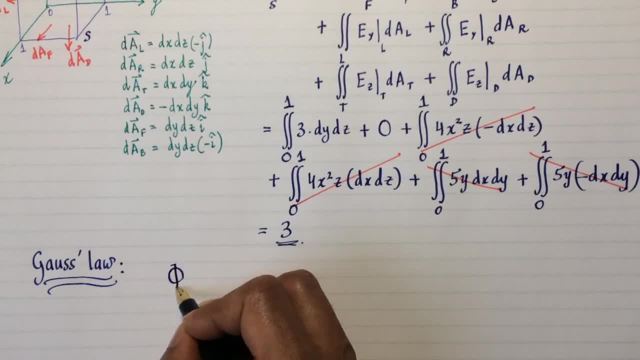 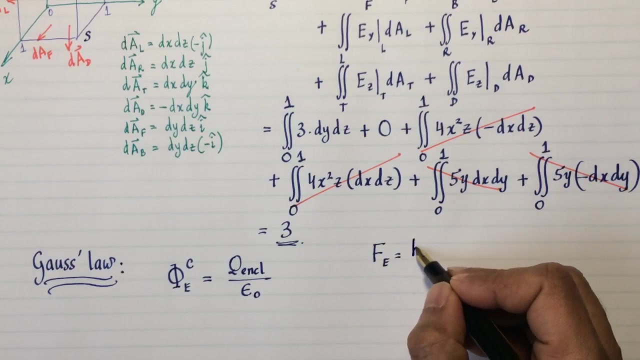 Gauss's law says the following: The closed flux is equal to the charge enclosed divided by epsilon naught. I have introduced epsilon naught earlier in week 2.. If Coulomb's law f, electric can be written as K, Q, 1, Q 2 over R. 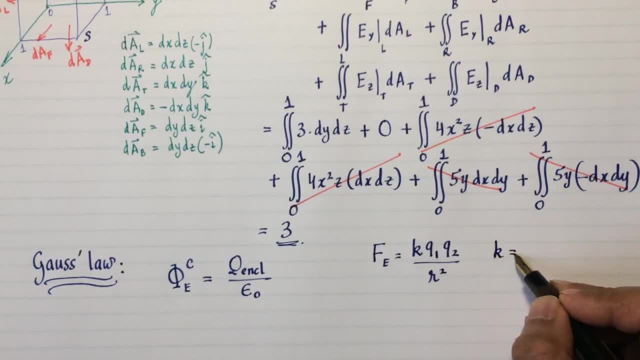 squared in magnitude, epsilon naught is related to the Coulomb constant K as follows: Coulomb constant K is one over four pi epsilon naught. So the value of the Coulomb constant, as you know by now, is 9 times 10 to the 9. 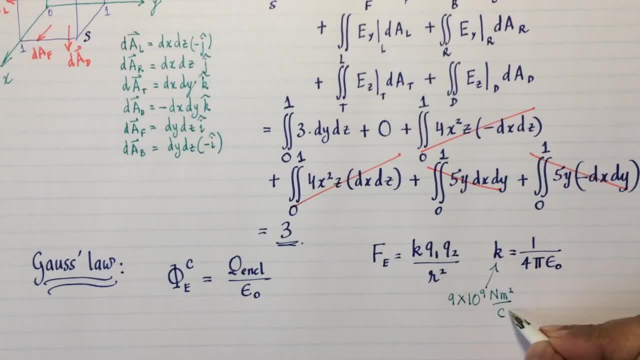 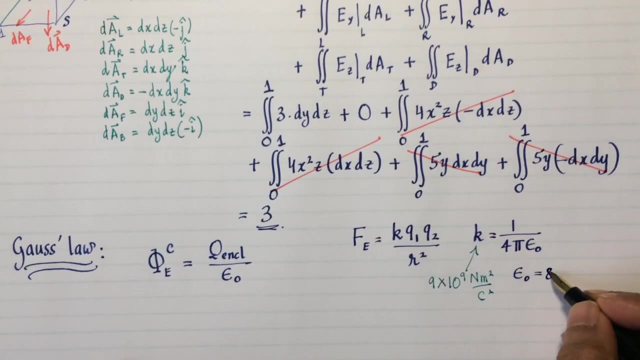 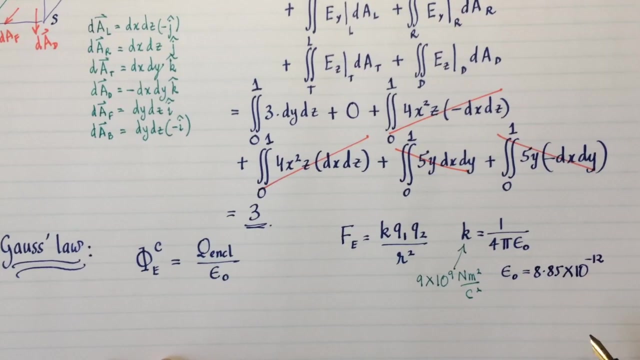 Newton meters squared per Coulomb squared. So epsilon naught can be worked out from that. If you work this out, epsilon naught is going to be something like 8.85 times 10 to the minus 12, and the units are going to be the reciprocal units of K, which don't really 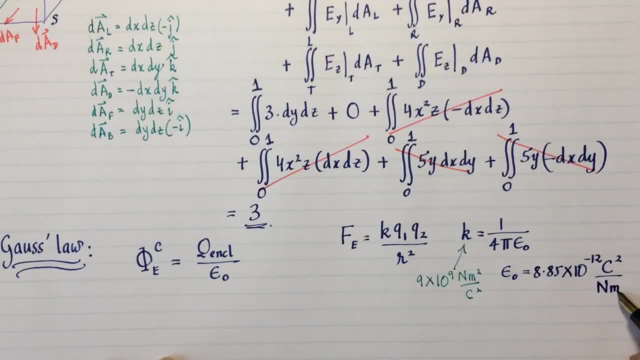 look good at this point, but later on we'll have far better units to give epsilon naught. In week 4, towards the end of week 4, I will give you some much better looking units- for epsilon not, but right now. let's just take the. 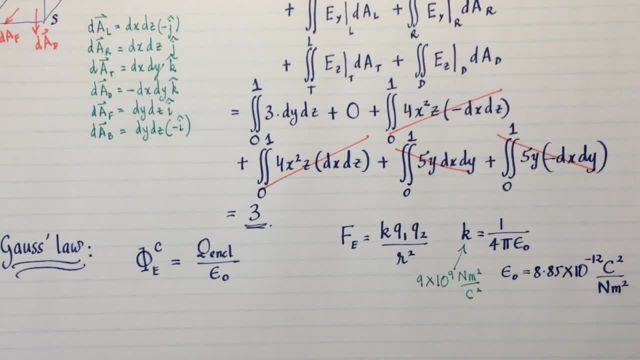 units to be those of 1 over K. So that's just a number. it's a number of the constant of nature, and there are experiments to measure it. What Gauss's law tells you is that the enclosed charge can be found once you find the. 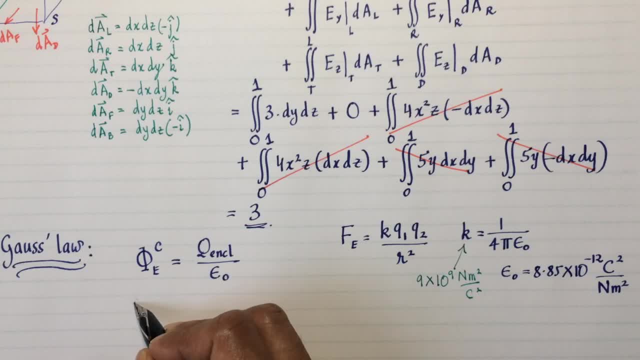 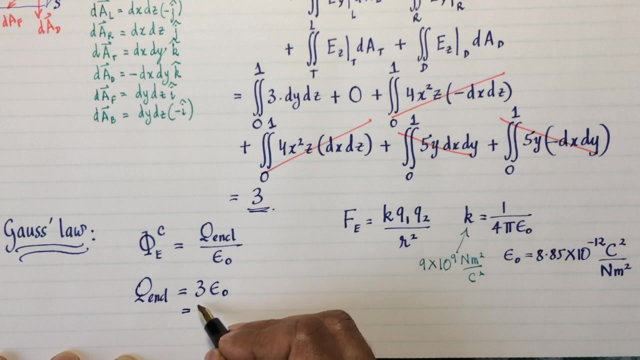 closed flux. So the answer to how much fish you've caught is really this: The enclosed charge, and the answer will be in coulombs. So it's three times epsilon naught. So I can basically do 8.9 times 3.. So 9: 3's are 27.. So this will be. 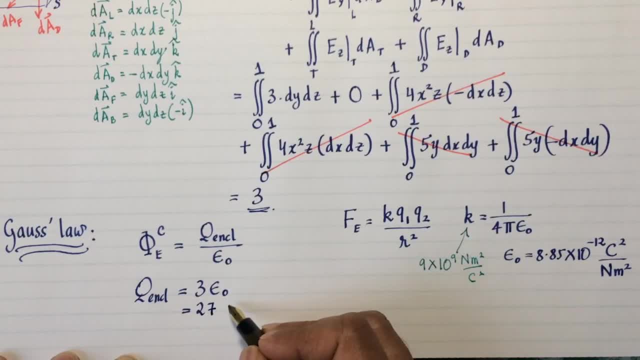 something like 27 times 10 to the minus 12 coulombs, or 27 pico coulombs, because pico is 10 to the minus 12.. In this manner, I've found out how much charge there has to be in the cube- by simply working out the. 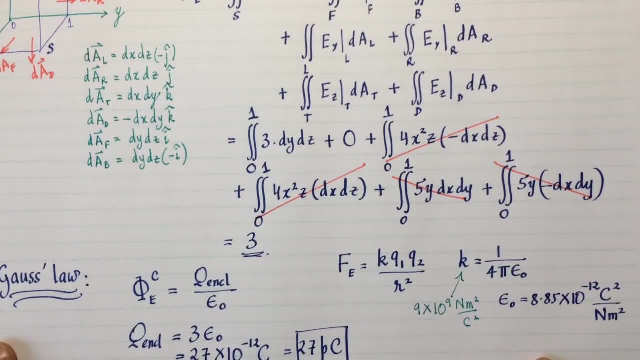 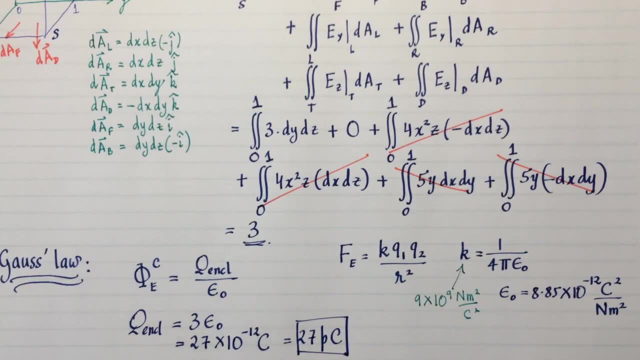 contributions of the electric flux on each surface of the cube. It's pretty remarkable that information on each surface of the cube gives you how much charge there is inside. It's as though you put the net inside the river and just look at the photograph, those surfaces and see how much. 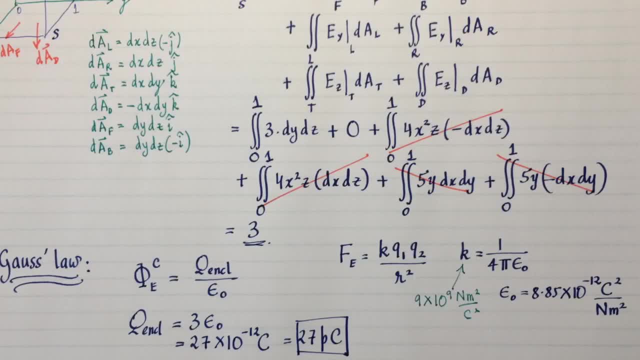 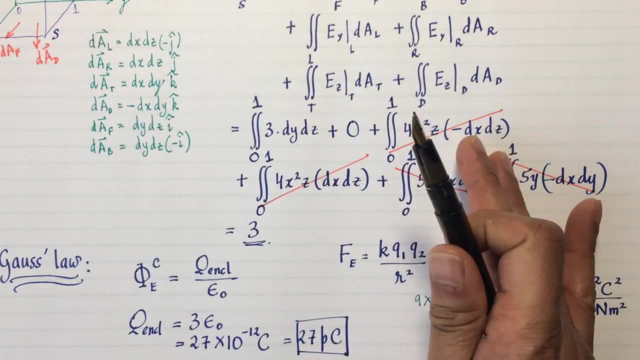 fish are darting in and out and into some surfaces you will find more fish coming in than going out and other surfaces you will find equal number of fish coming in and out. these two surfaces that cancel surface contributions that cancel are those fish that simply come in the one surface and 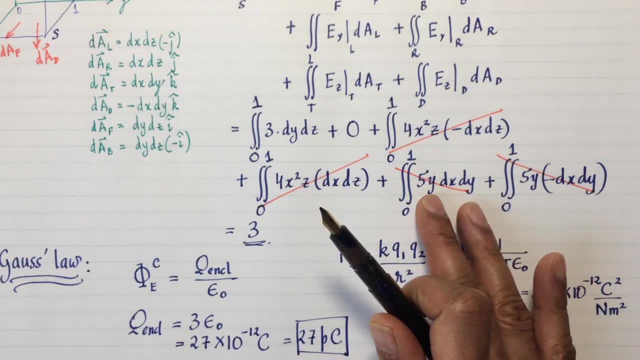 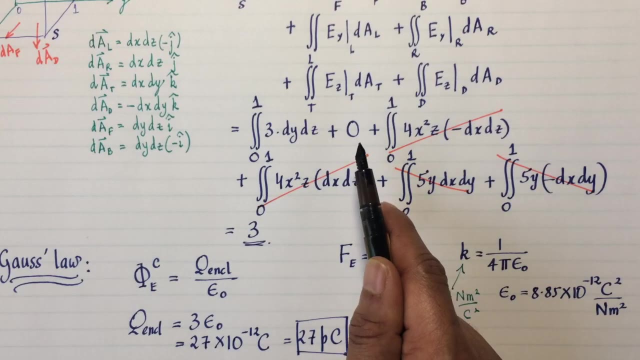 exit the opposite surface. same thing with the fish in the Z direction. they just go in and in one surface and come out the other surface. the only fish that get different counts is in the. in these, these two terms, in the front and the back, you'll find that no fish are coming in from the back, but fish are coming out.